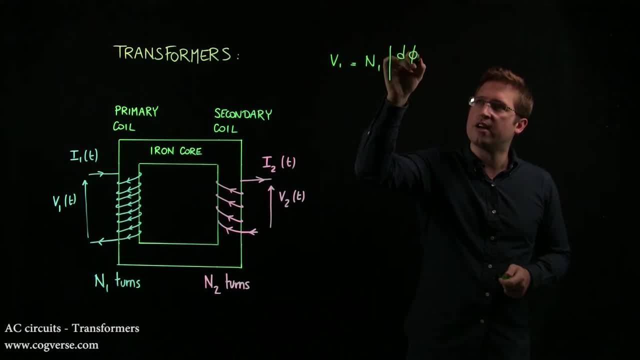 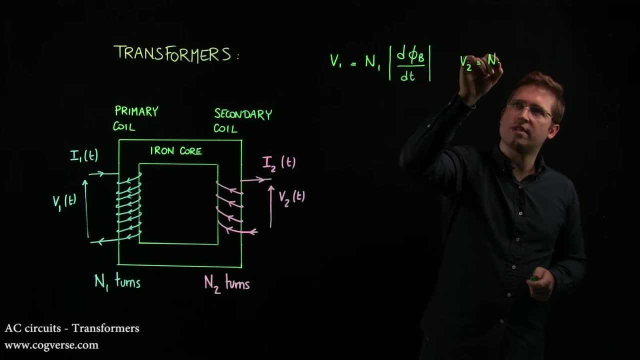 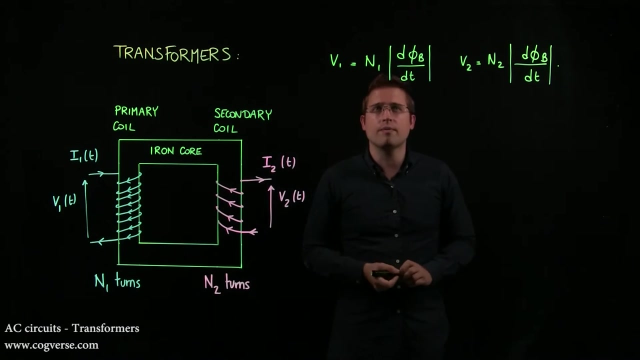 is equal to N1- absolute value of d phi b over dt, And V2 is equal to N2- absolute value of d phi b over dt. But these two quantities are the same again because the magnetic field lines are trapped inside the iron core. So 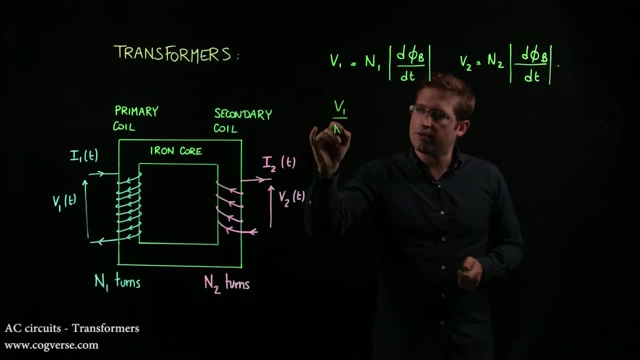 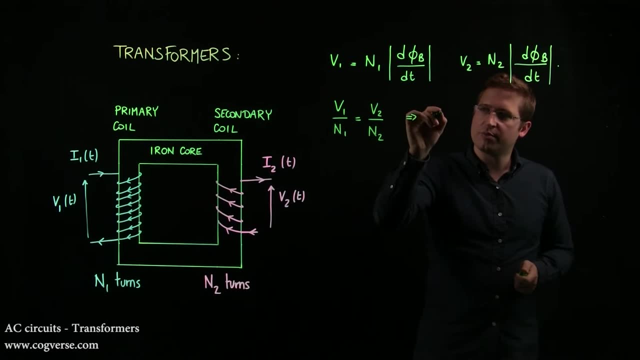 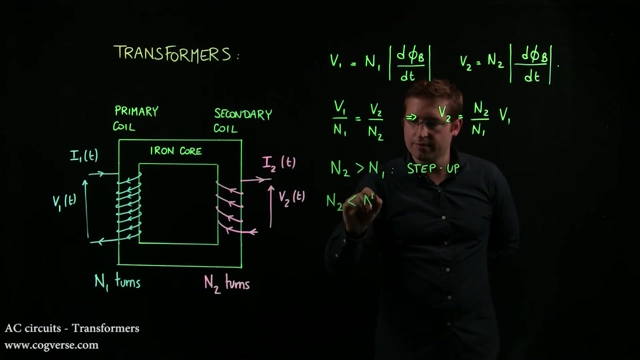 we can write that V1 over N1 is equal to V2 over N2.. So we should write V1 over N2.. So we need: V2 is equal to N2 over N1, V1. And if N2 is greater than N1, then you have a step up transformer. If N2 is less than in N1, then 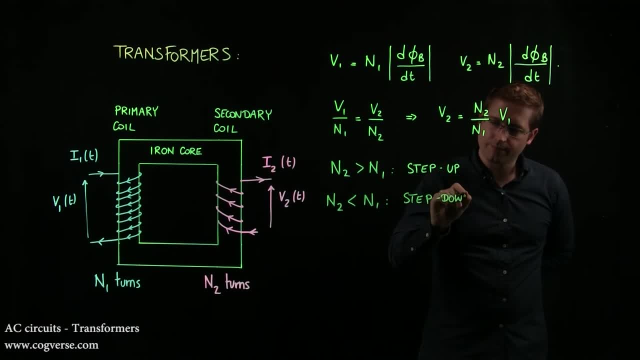 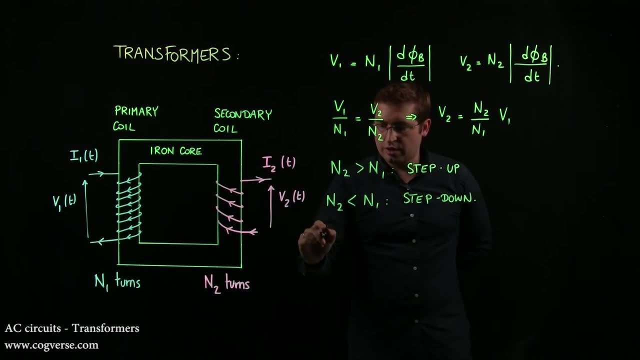 you have a step down transformer And if you have an ideal transformer, then you have an ideal transformer and that transform. and again it turns out that the spaced müsste of a transporter versus a respect to an ideal transformer. if there are no power losses, you can also write that P1 is equal to 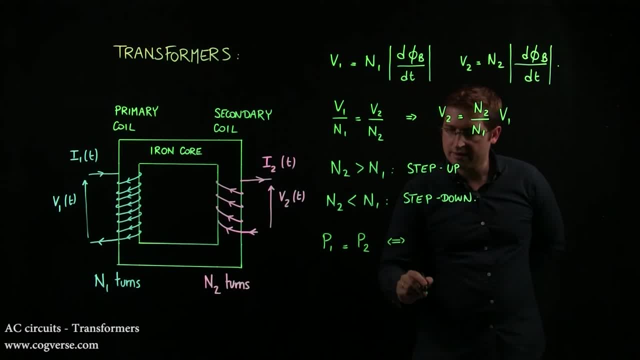 P2, and that tells you that V1, I1 is equal to V2, I2.. In other words, that you can relate I2 to I1 through the ratio N2 over N1, because we know that V2 over V1 is N2 over N1. So we have: I1 is equal to V2 over V1, but that's N2 over N1. 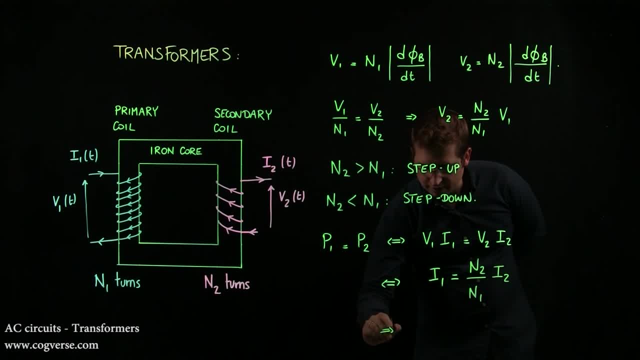 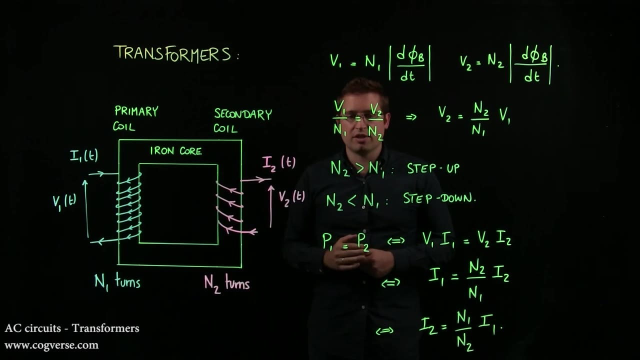 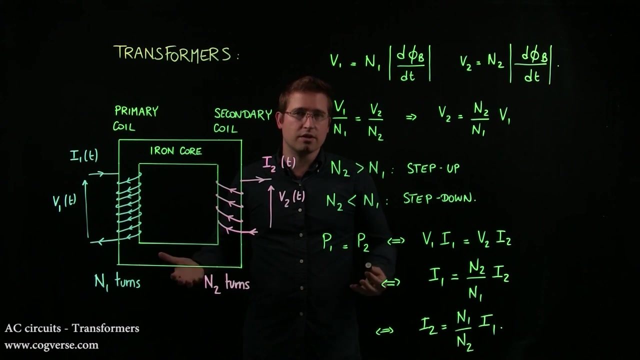 x, I2.. And finally you get that I2 is equal to N1 over N2, I1.. So that's the idea behind transformers. It's an induction based component, and so it only works with AC voltages and AC currents, because you need a varying magnetic field here to induce a voltage across. the secondary coil.